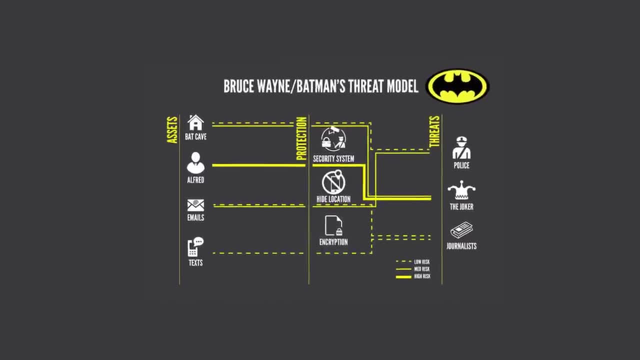 to be talking about today. I'm going to be talking about how to protect yourself against what they call threat modeling- in security, I guess- And basically for this video we're going to limit ourselves to, you know, stuff like stalkers, hackers, vindictive ex-partners. 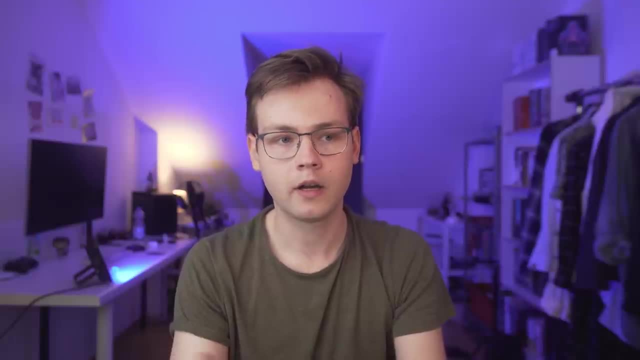 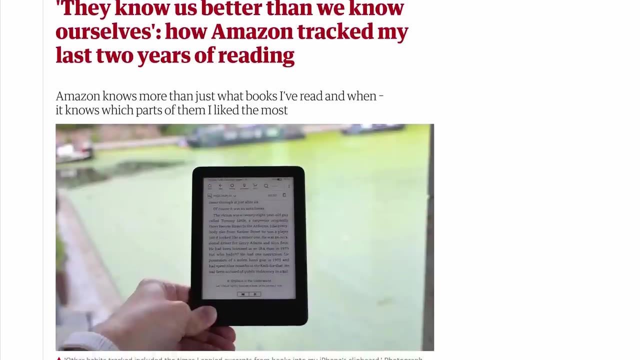 basically people and companies who want to leak your personal data, whether by choice or by mistake, that doesn't matter. We are not, however, going to cover mass data collection that is performed by companies like Google, Amazon, Microsoft and Apple. This is a little bit. 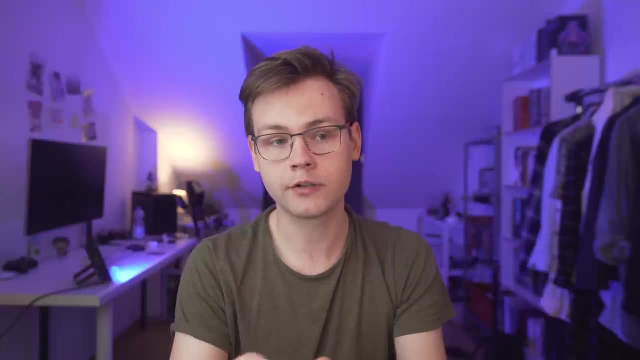 more complicated and a bit out of scope for this video, So we're going to limit ourselves to a scenario in which you are individually targeted. And last thing I want to mention before we actually start with the tips is that none of the companies or services that I mentioned- 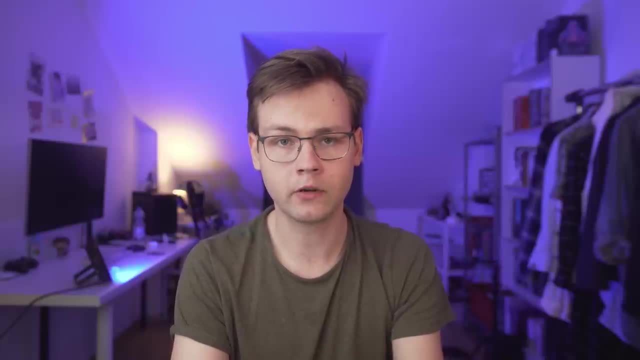 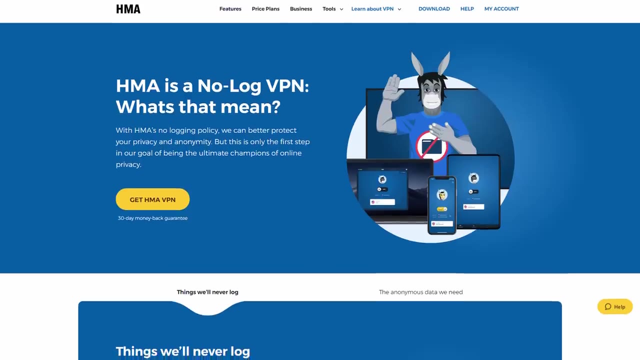 in this video paid me or somehow sponsored this video. I'm also not paid by FBI, CIA, KGB or any other you know three-letter agency to shit talk VPNs and other services and applications that are useless for privacy. I do it for free, swear to God. Now, on that note, 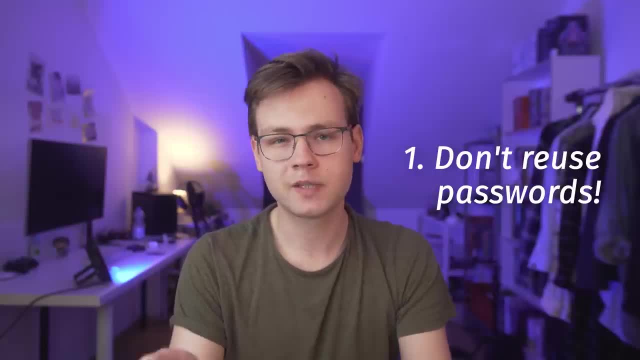 let's start with my first tip, and that is: do not reuse passwords. It's a pretty basic and obvious tip that I think everyone is aware of, but please take it seriously and do not ever use the same password for two or- you know- multiple services. That is especially relevant with small. 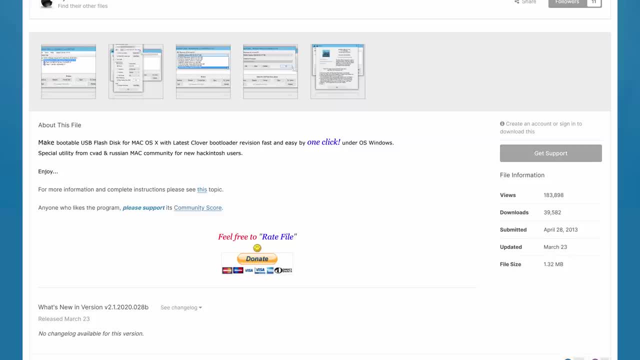 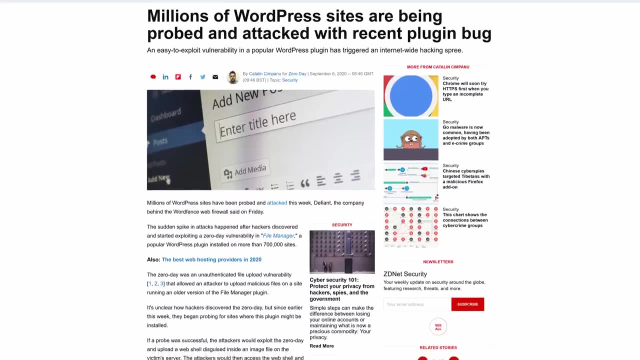 websites or, just, you know, forums that you register on just to download one file or something to that effect, because those websites are very likely to get hacked at some point, Especially with those smaller websites and forums. what can often happen is that their website gets. compromised on some level and the database with all the users gets leaked. And if they're storing your password in plain text- which is you know you're not supposed to do that, but some people do that anyway- your password will basically now be available to any 13 year old lead hacker teenager. 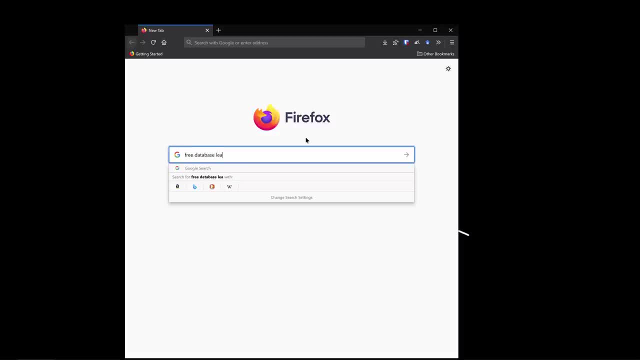 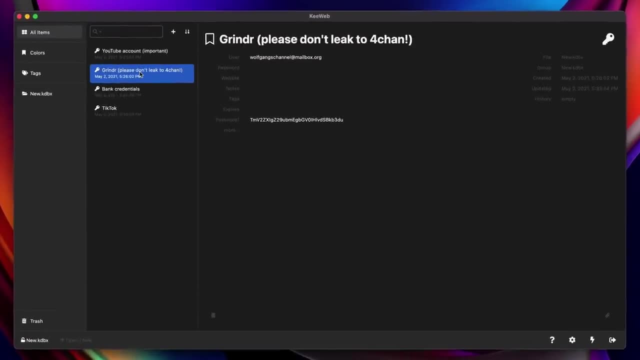 who has enough. you know Google skills and can just Google stuff. like you know. password database 2021.. Trust me, you don't want to take that risk, so please use a password manager. I know that it can be pretty tedious and annoying to just go through all of your. 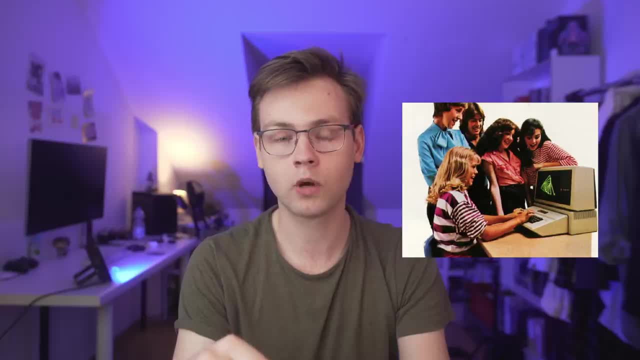 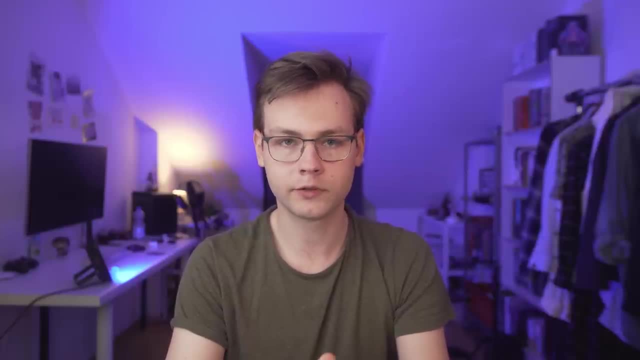 accounts and change the password everywhere, especially if you're like me, if you grew up with internet and didn't exactly follow the best security practices as a teenager. but trust me, it's definitely worth it. You just don't want to take this risk. 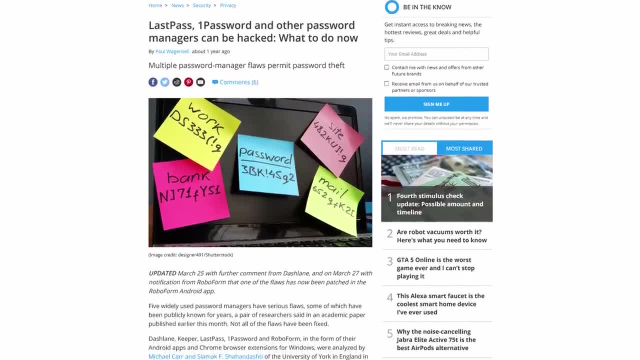 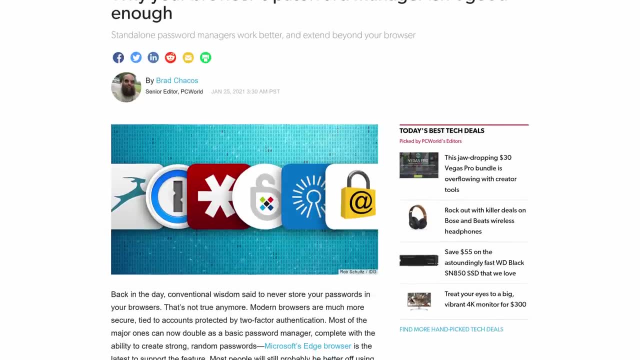 As to which exact password manager I would recommend. I would definitely advise against using cloud-based solutions like LastPass, or even just using a password manager that is built into your OS or your browser, such as Chrome, password storage or Safari, because a password database 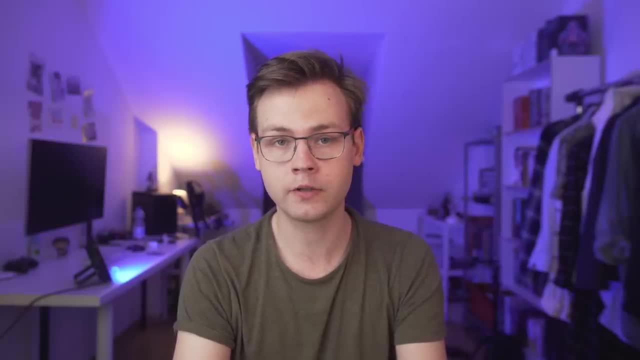 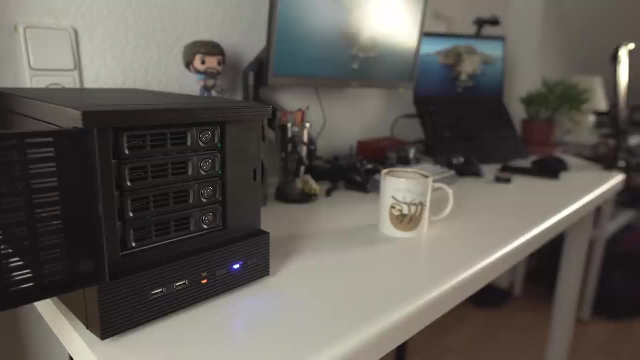 is a very, very, very sensitive information that you don't want to put in the cloud. You want to have full control of it. So that means either having it on your local machine or having it on a self-hosted home server, but that's a little bit more advanced. So if you want to go the simple route, I would recommend KeePass. KeePass is basically an open source standard for password databases. You can store them locally. There's a lot of good and open source clients on basically every operating system imaginable. 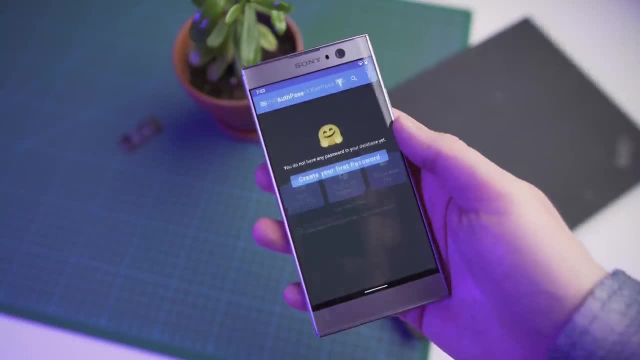 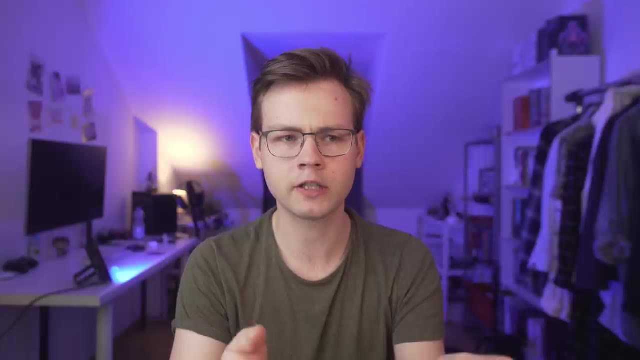 so Windows, Linux, macOS, Android, iOS, what have you? However, if you have multiple devices which you use to log into your accounts, it can be pretty annoying to basically juggle the KeePass file, you know, back and forth. 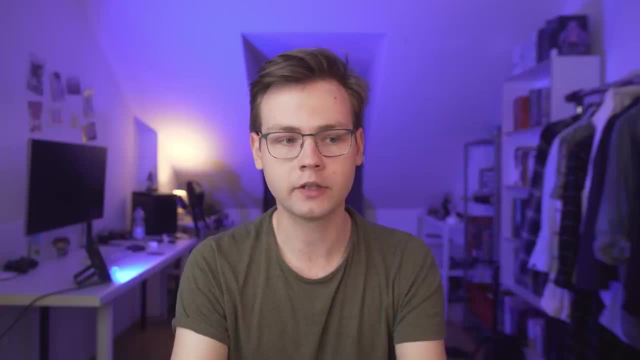 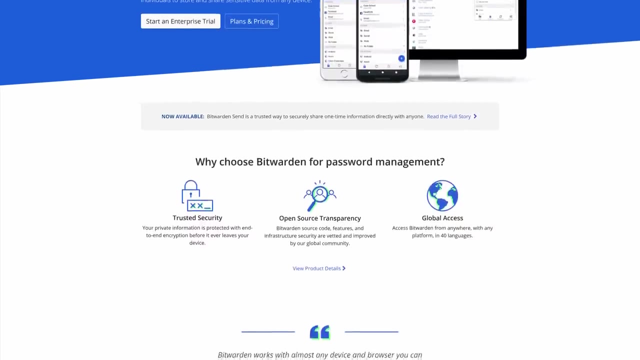 So if you have something like a home server, for example, or a NAS, you can basically self-host a Bitwarden instance. Bitwarden is an open source password manager and you can basically self-host it on the premises. And yes, that technically means. 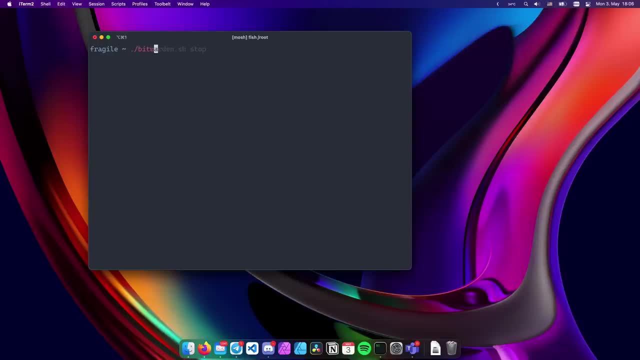 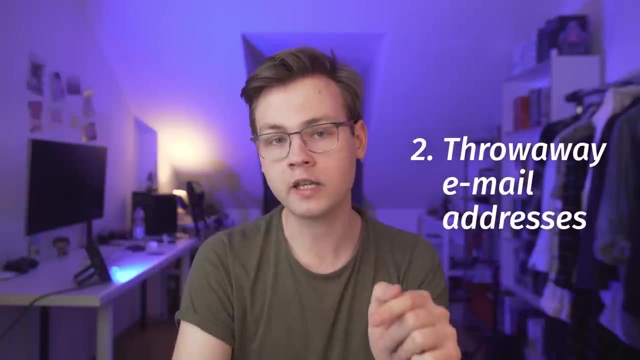 that you will be storing your password database in the cloud, but this cloud will be your own home server in your own house, So at least you have some degree of control over that. The next tip is: use throwaway email addresses and also alternative emails. 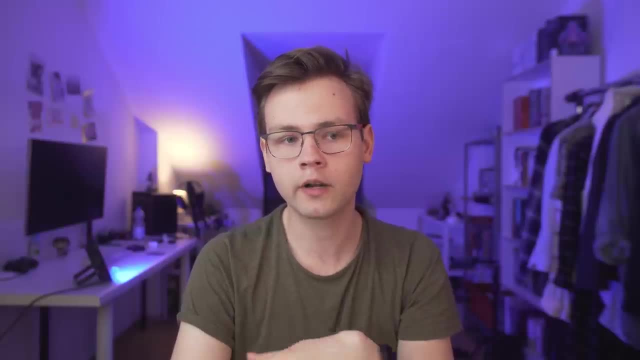 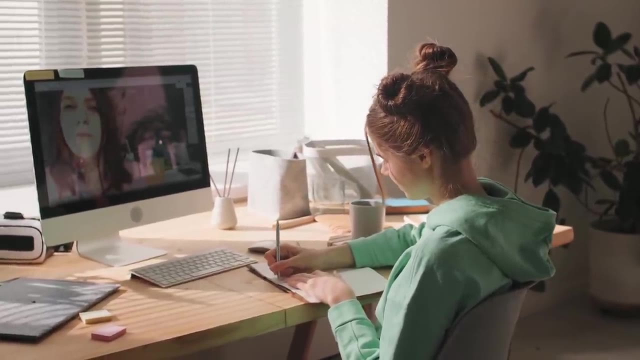 The reason is basically, if you use one email address to log in everywhere, you will be very easy to identify. For example, let's say you use email address, one email to log into like school, like online platform, and the same email to log into- I don't know- My Little Pony forum or something. 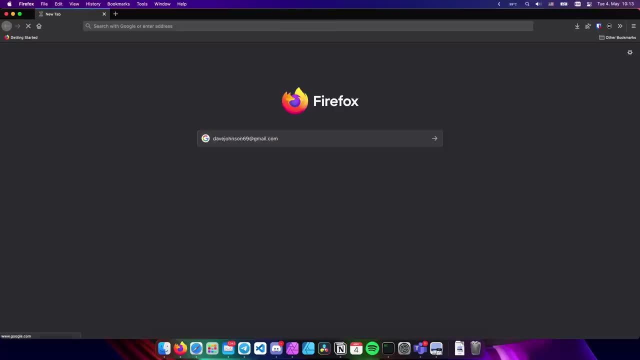 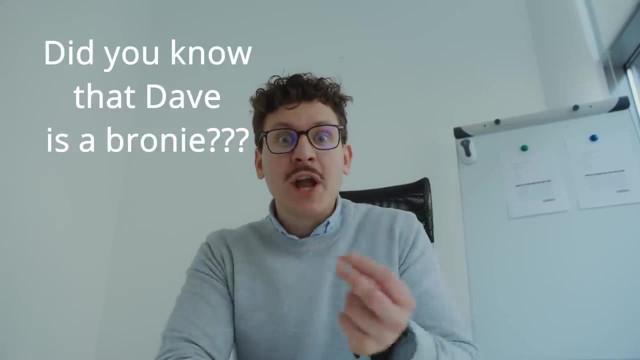 And if your classmates Google your email address, they will most likely find your account on that, My Little Pony forum, and that would make for some embarrassing conversations in the Zoom breakout sessions. I guess It's a pretty stupid example, I agree, but I think you can. 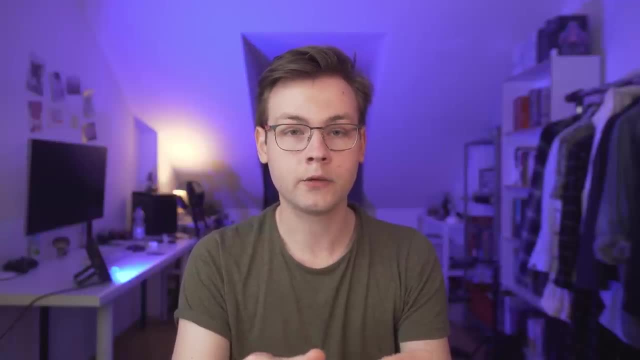 imagine what can happen and what someone can do if they have your email address and you use this email address for basically everything online. So don't do that. If you have an Apple account, a lot of services now support logging in with Apple and there, basically, Apple gives you an. 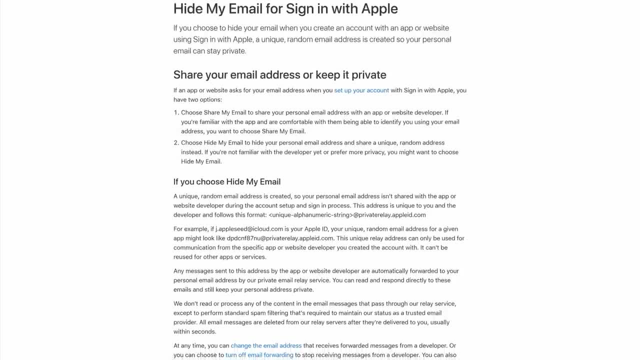 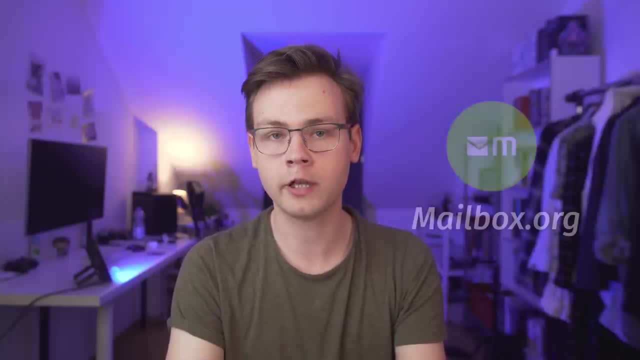 option of hiding your real email address and replacing it with an anonymous, randomly generated email, So you can use that. Alternatively, if you're not a fan of Apple ecosystem, there is a service called mailboxorg. This is what I basically use for my personal email. 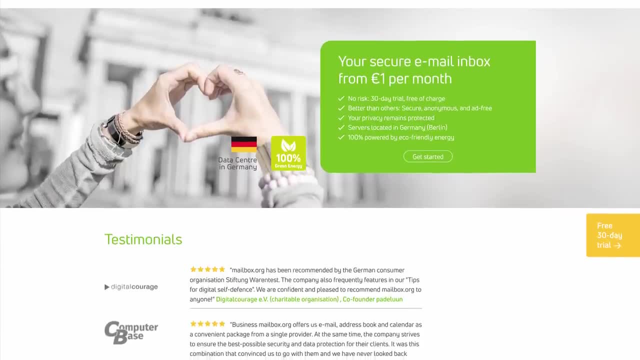 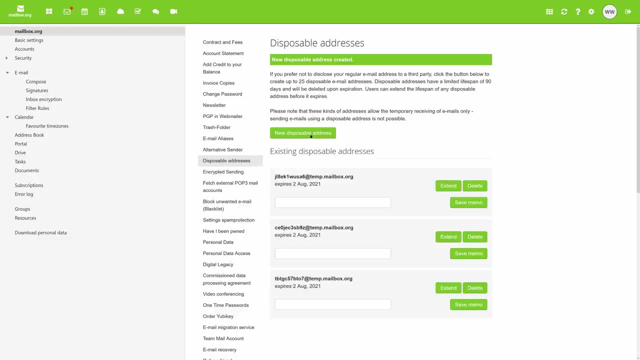 There you have an option of creating 25 aliases for all of your different email and account needs, And they also provide an option of throwaway accounts. So if you need to sign up for a giveaway or something similar, but you just want to have a possibility of just clicking on X and you know, deleting this throwaway email address. 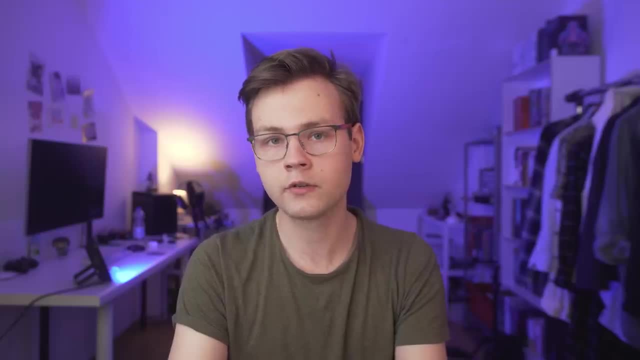 and not receiving anything on it ever again. It's not free, though. The tier that I'm using costs three euros, but I think it's worth it, considering you know the functionality that I just mentioned. So, yeah, And then sometimes you just need to enter an email once and you. 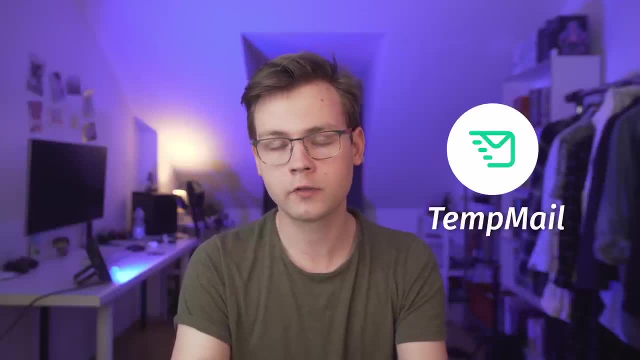 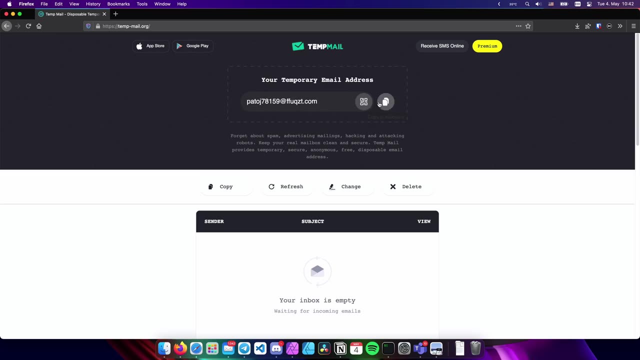 never want to be contacted by a company ever again. For that I'm using a service called tempmailorg. This service basically gives you a random email address which you can use to receive one or maybe a few emails, and then just close the tab and 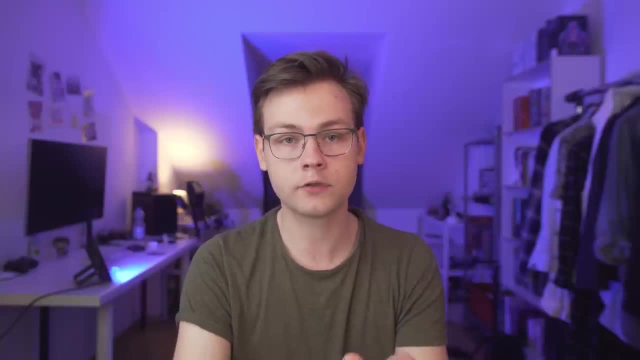 poof, it's gone. There is no identifying information. You don't have to supply your personal email, So that's something I use a lot for those shady services that I don't want to. you know, give my actual email address to. 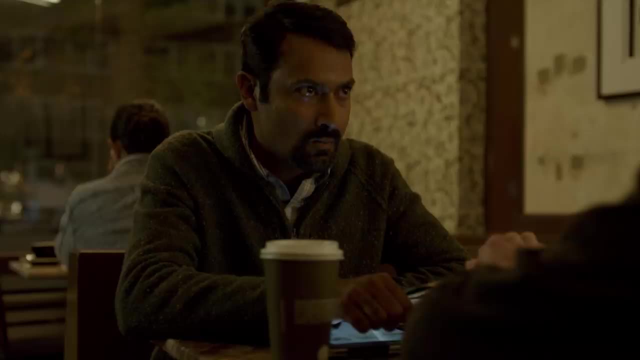 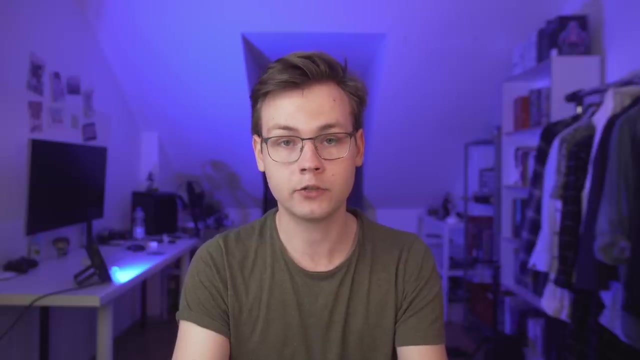 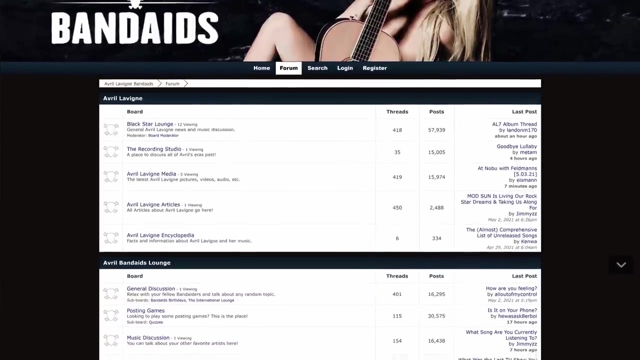 My next tip is clean up your older accounts. Sometimes people don't realize how much personally identifiable and sensitive information one can find about someone after just typing their nickname into Google. If you're curious, just do it yourself. Type your nickname into Google and you'll probably see a lot of you know stuff from your teens accounts on. 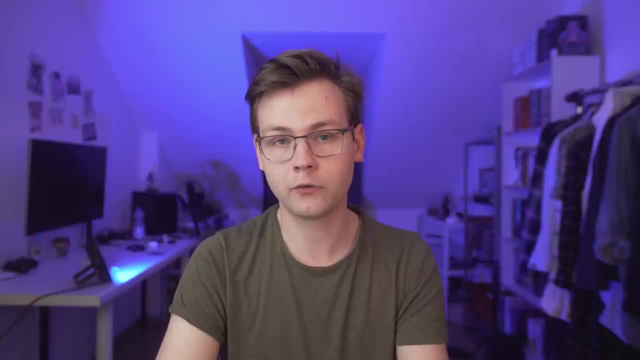 gaming websites, forums and stuff and so on and so forth. So my recommendation is go on Google or DuckDuckGo or whatever type your nickname or your full name and see if there are any like accounts, any traces that you left online that you don't want to be there anymore. Sometimes that's 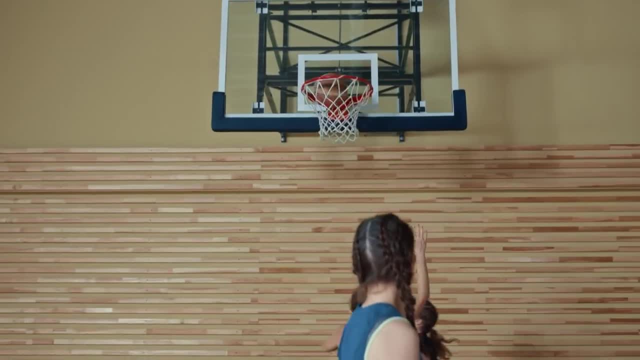 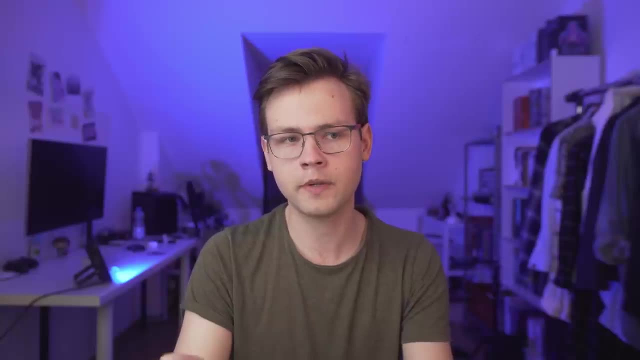 obviously out of your control. Sometimes you know there are schools that post athletic records online, or maybe other companies would post stuff about your online that you can't delete or modify. But for everything else that you can control, just make sure you go over all the accounts. 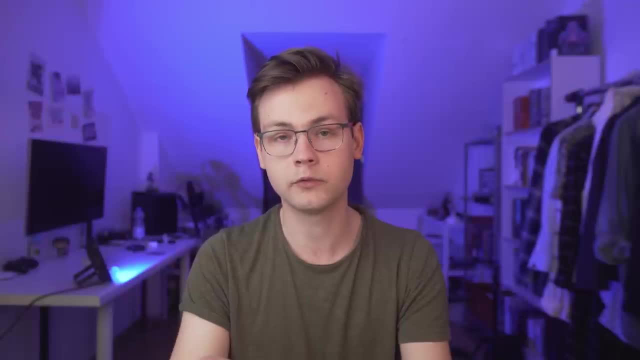 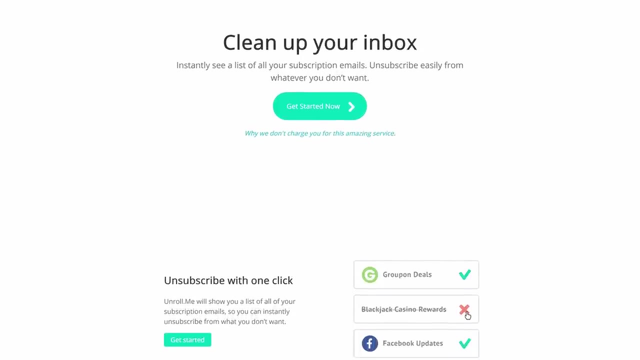 all of your old stuff and just clean up stuff that you don't want other people to find. You might be very tempted to use a service like unrollme, which basically goes through your email inbox and, you know, sees if there are any. 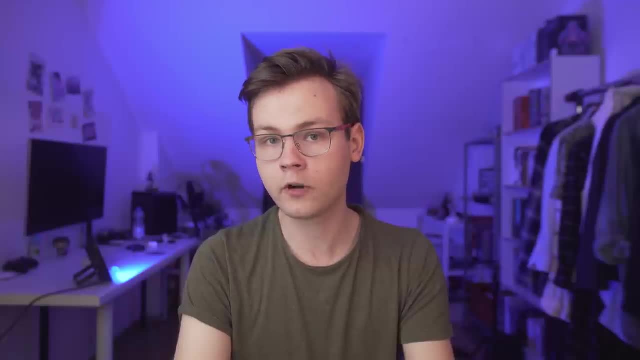 services, websites or newsletters that it can unsubscribe you from. But I would advise against those services because you practically give them full access to your email inbox to all of your messages. In my opinion, that's just never a good idea because you don't know what they're. 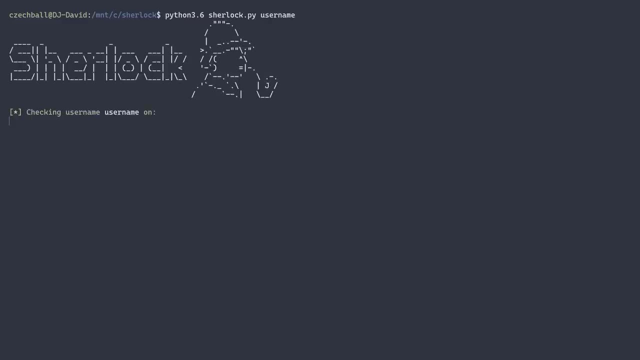 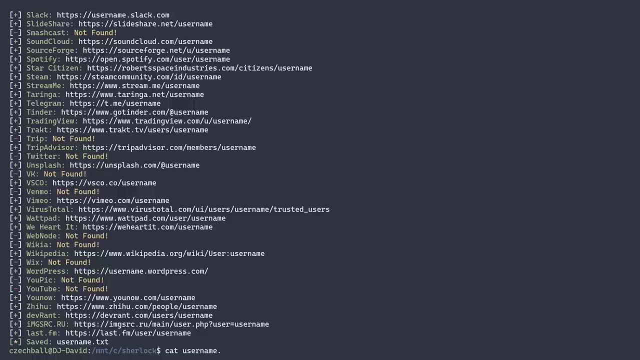 going to do with your messages. Instead, there's an app on GitHub called Sherlock, which you can basically use to look up people's accounts online on like a lot of websites, including Facebook, Twitter, GitHub, Tinder, ResearchGate, 9gag, And you can use it to look up your own nickname. 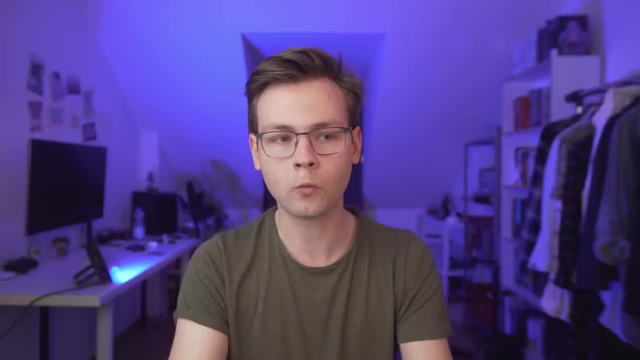 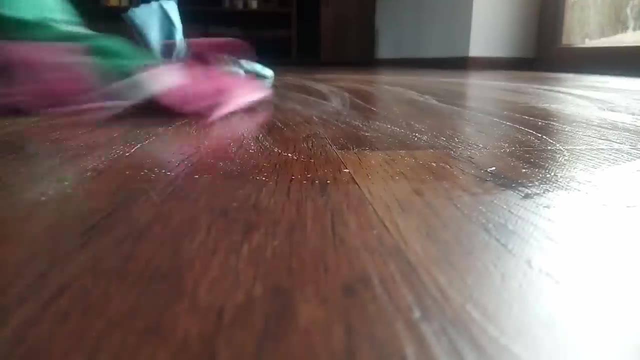 and see if there are any undesirable accounts that you don't want people to find anymore. Next tip that is kind of related to the previous one is use a random nickname whenever you can. As we all know, the best way to clean up is don't make a mess in the first place. So if you don't, 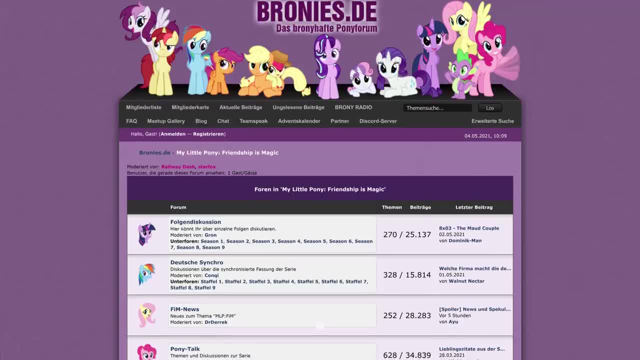 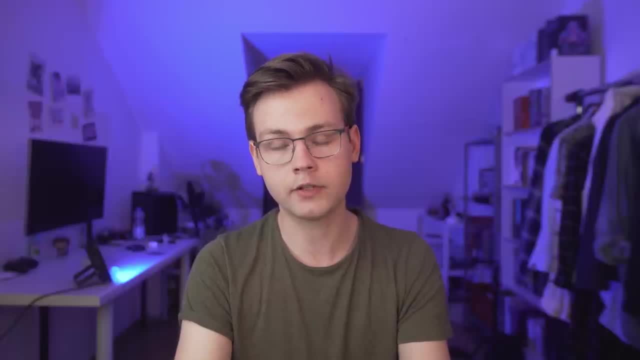 want to have to do the same thing with Googling your nickname and deleting old embarrassing accounts five years from now. you should use a random nickname every time you can. Your nickname can obviously identify you and help the attacker find more information about it, So you should. 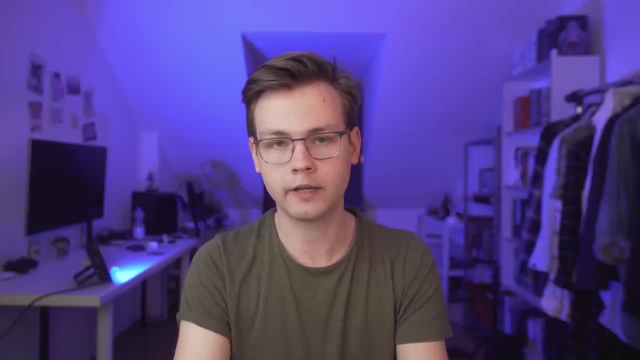 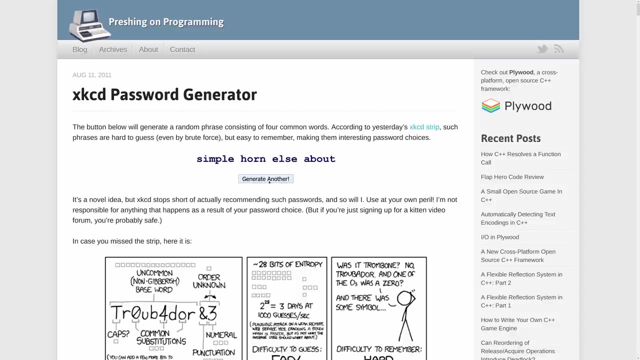 definitely avoid using one nickname for every service. online, You can use XKCD password generator. This will basically help you create a random rememberable string of letters that you can use as your nickname And then, if you have trouble remembering all of your random nicknames, 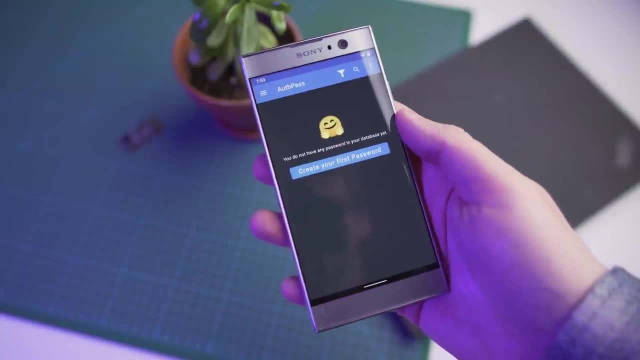 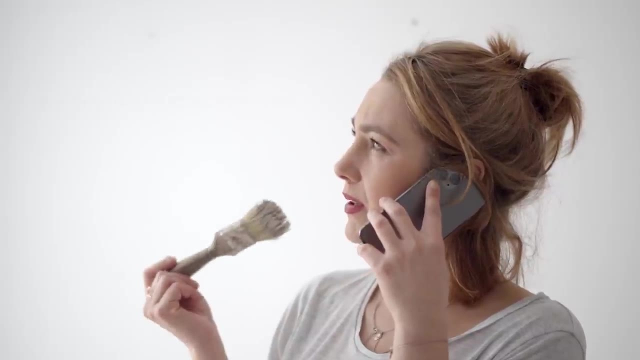 you can use password manager to put them all in Very convenient. My next tip is: don't give away your real phone number. Your phone number is something that you don't change very often because it's a pain in the butt. You don't have to change your real phone number every time you use it And you usually keep a phone number for years on end And because of that, a phone number can easily be used to identify you. In some countries, there are illegal services that basically give anyone access to a database which matches phone numbers with full names and 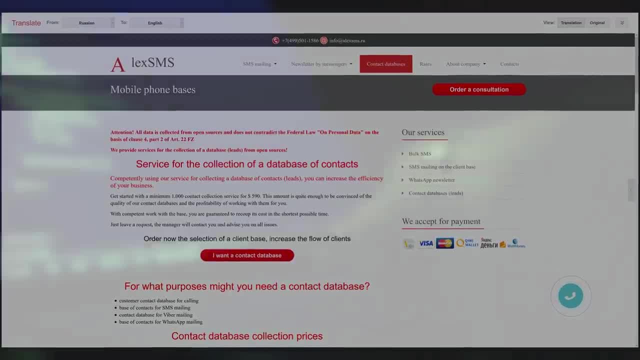 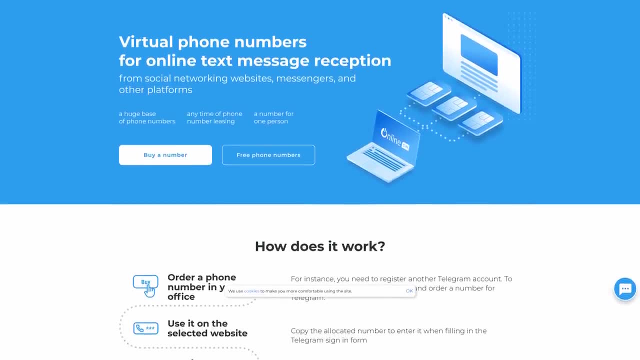 addresses, So be sure you don't give your phone number just like that online. Instead, I would recommend using a virtual number service like this one. This is online simru. Yes, it's a Russian one, but it does have an English version. The costs on this particular website are super low. 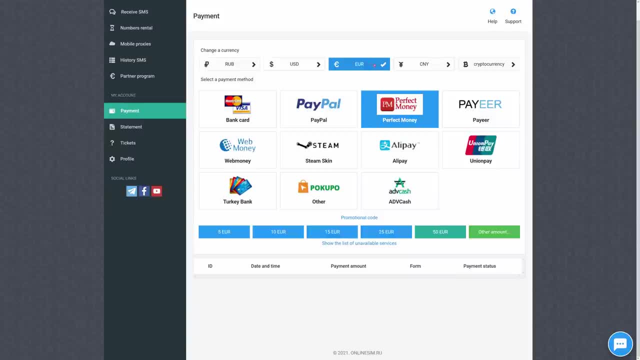 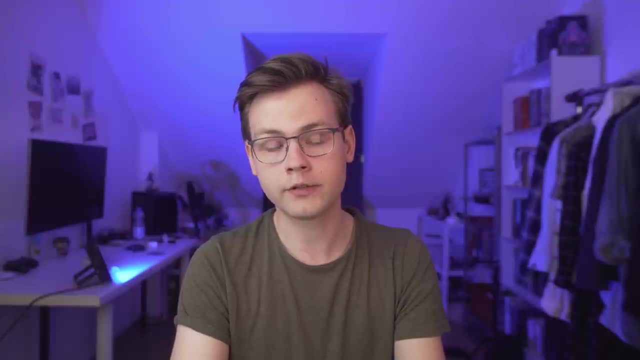 You can basically get a number for as little as five cents. You can also pay with crypto, so Bitcoin, Ethereum or anything like that- but those numbers are basically one time use. You can use them to verify your Telegram account or your Discord account, but it's not going to work for something like WhatsApp or Signal. 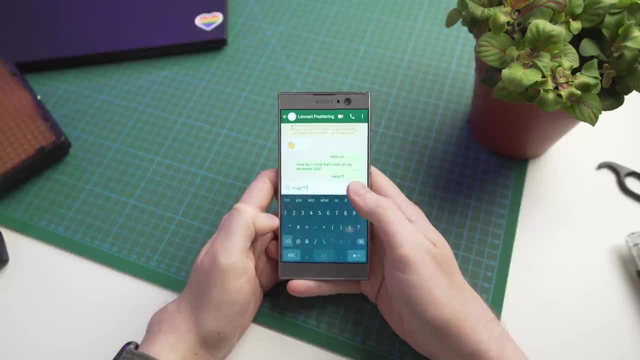 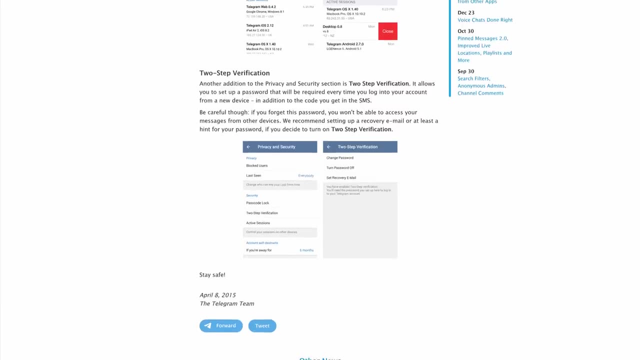 We need to have the constant access to the number So you know, in case you change your phone or lose it, you can re-register the accounts on the new phone. Also, if you're using a virtual number for Telegram, make sure to set a number password so that you won't basically give full access to 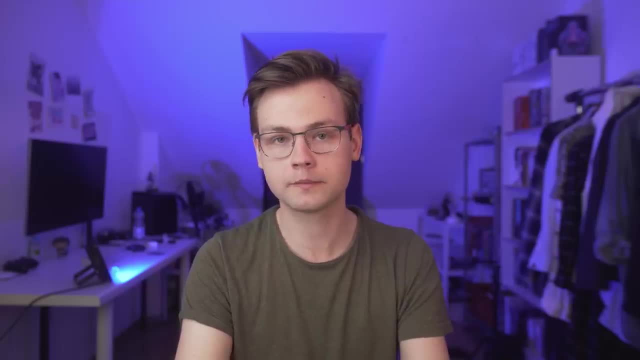 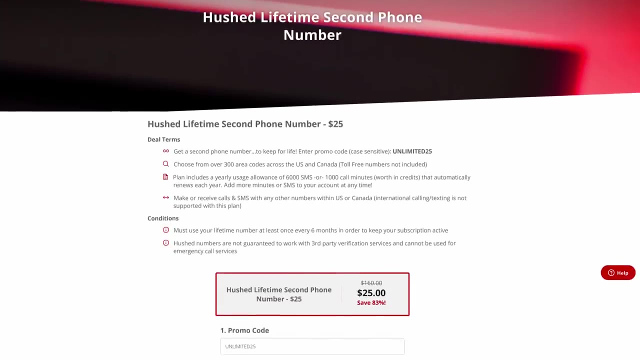 all the messages to anyone who tries to register with the same number. As an alternative to apps that you need number with often, for example, WhatsApp or Signal, there's a company called Hushed and they offer a lifetime access to a virtual phone number for. 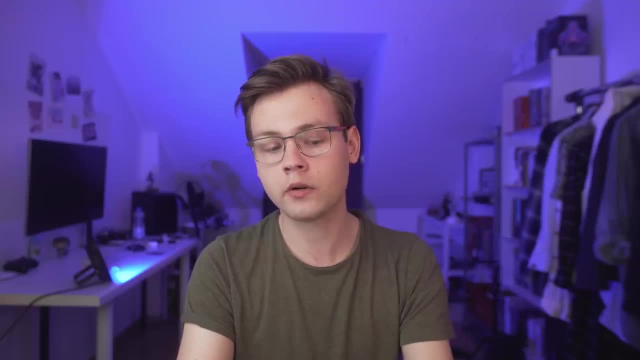 as little as, I think, 40 bucks. You can only pay with credit card, though, and you have to put your real name. And then also, if you don't use this number for a while, they will deactivate it, which sucks, You know, it's not actually lifetime. And while we're on the topic of phone, 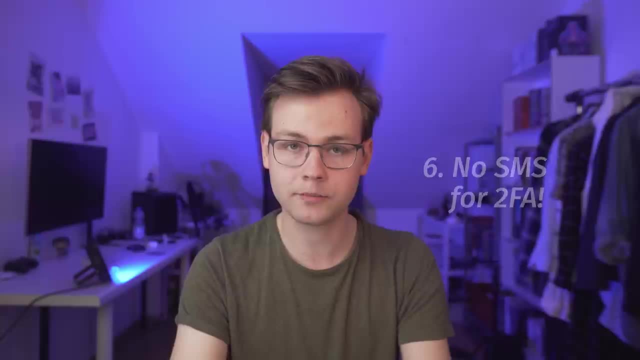 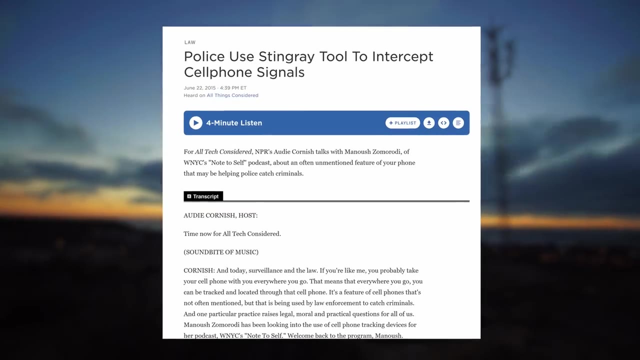 numbers. do not use SMS for two-factor authentication. First because it will require you to give your phone number duh, And second, because SMS messages travel unencrypted and can be intercepted by police or a bad actor. And then third. in some countries, the bad actor can pretend to be you, call the cell provider and basically request a new SIM card replacement for the same number. It is pretty illegal but not uncommon. Instead, you should use a two-factor authentication app on your phone, such as: 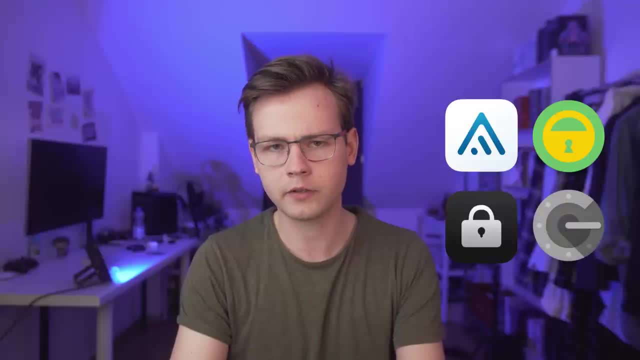 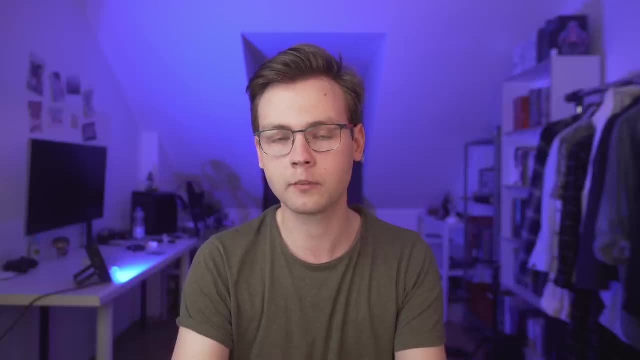 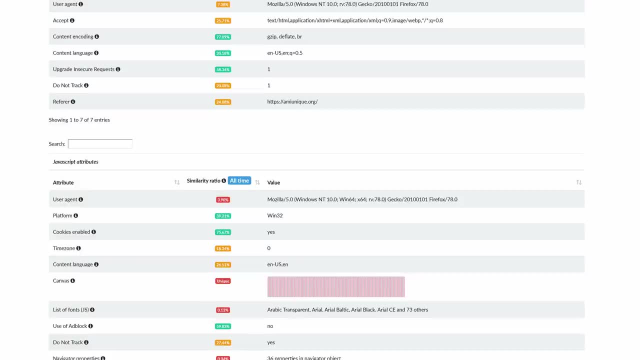 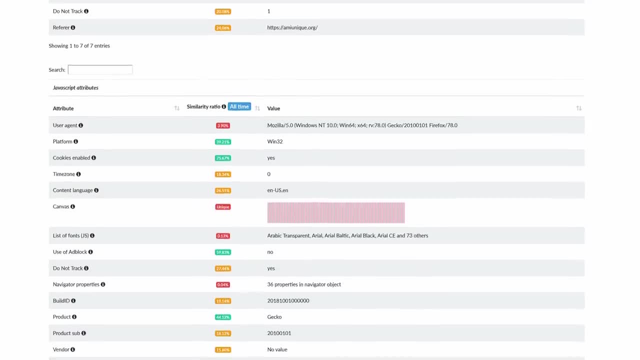 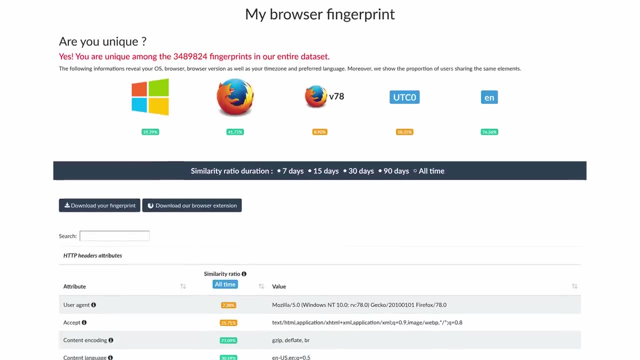 the extensions that your browser is using, the fonts that you have installed, and so on and so forth, And the more unique this information is, the more identifiable you are online. But you don't have to take my word for that. Just go to miuniqueorg and see for yourself Who needs IP address when. 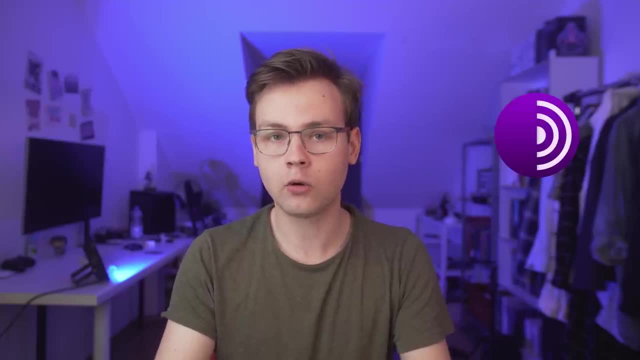 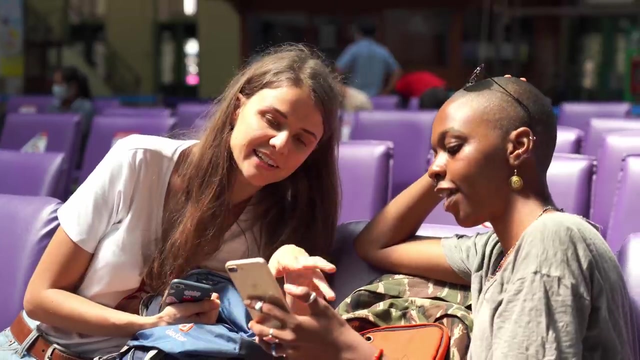 you have this. Is there a way out? Yes, Use Tor or Tails for super sensitive stuff. My next tip is basically compartmentalize, compartmentalize, compartmentalize. Make sure your online personas are separated. Use different email addresses and nicknames for stuff like school work, your personal. 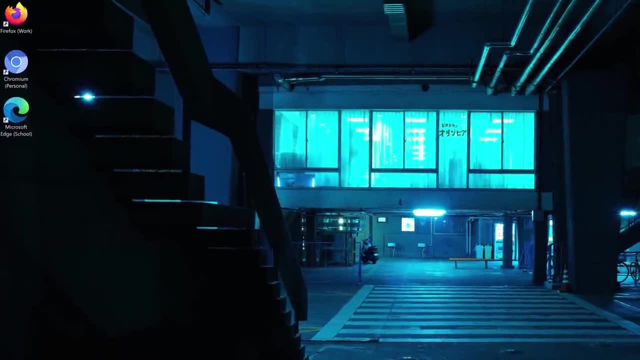 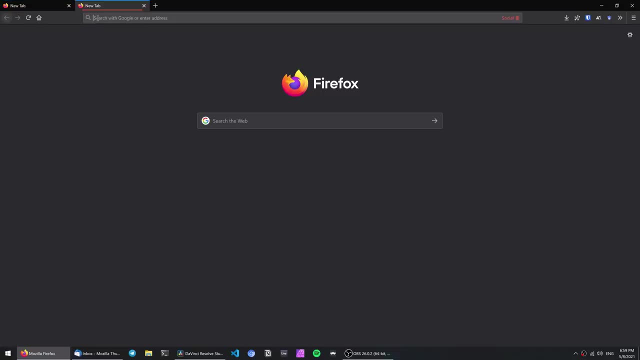 browsing and shopping And, if possible, also use different browsers or browser profiles. Firefox, for example, makes it very simple with an extension called container tabs. Basically, you can set some websites to open in containers which act as separate browser profiles. They can't read each. 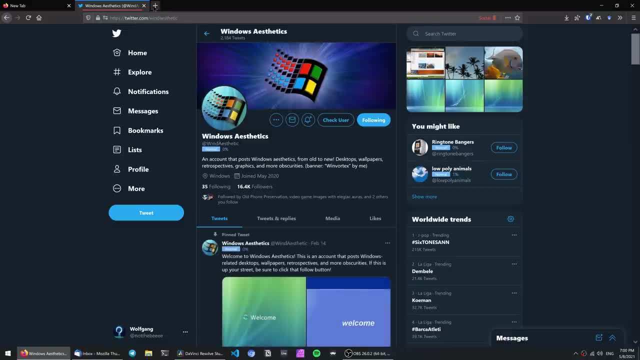 other's cookies, cache and so on. This is a very useful extension and it's one of a few resources that you can use to open up your browser profiles. So, if you're looking for a reason why I still stay on Firefox and not like Chrome or Safari, I've never met this man in my 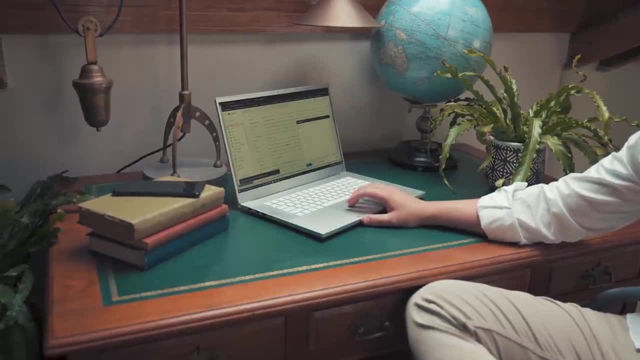 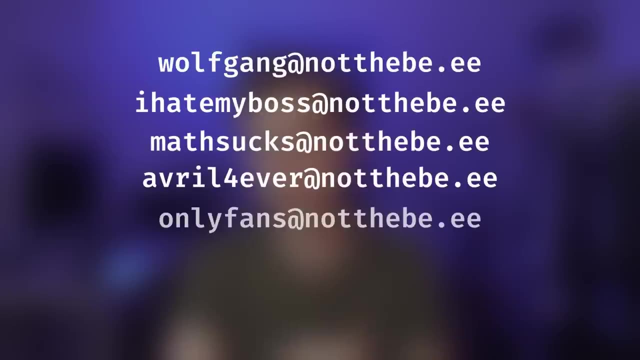 life, And I've already said it earlier, but I'm going to say it again: Use different email addresses for different stuff that you do online. Make sure you have a separate address for work, school, personal stuff, sensitive stuff for companies that you want to hear from from companies that. 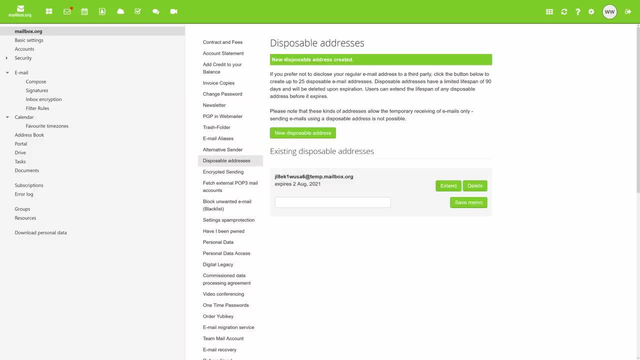 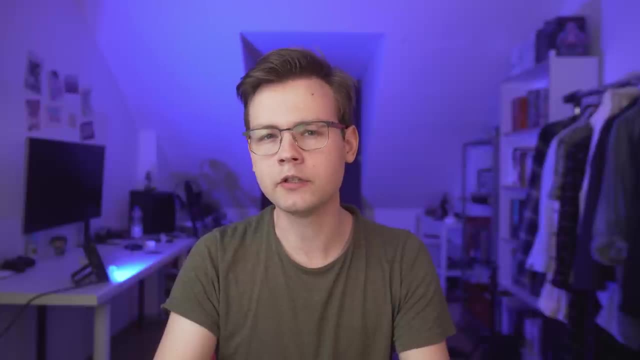 you don't want to hear from, The more the better. An email provider that has support for aliases, such as mailboxorg, can definitely help with that. And then, last but not least, there is a link in your privacy, but it's all going to be useless because you have that one friend or family. 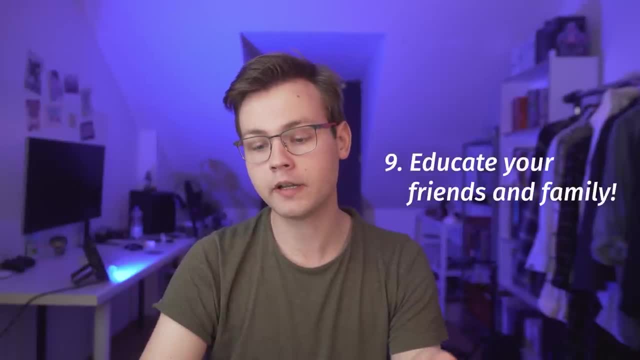 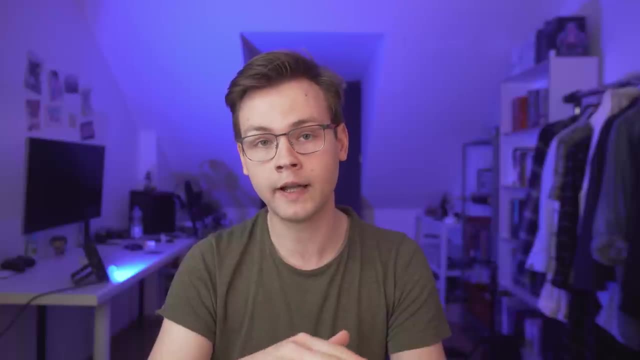 member that doesn't care about privacy. So my last tip for today is: ask your friends and family members to never, ever ever give any personal information about you to anyone online who would pretend to be your friend, your girlfriend, your ex-schoolmate, your doctor, your lawyer. 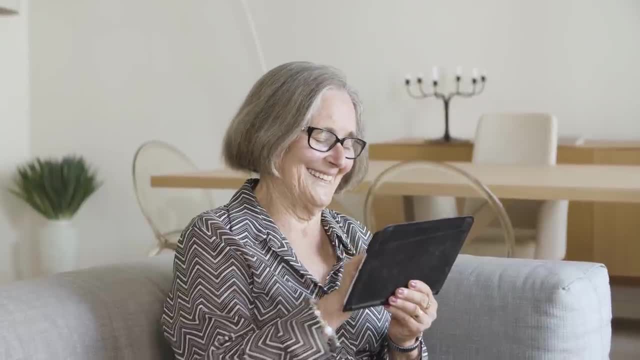 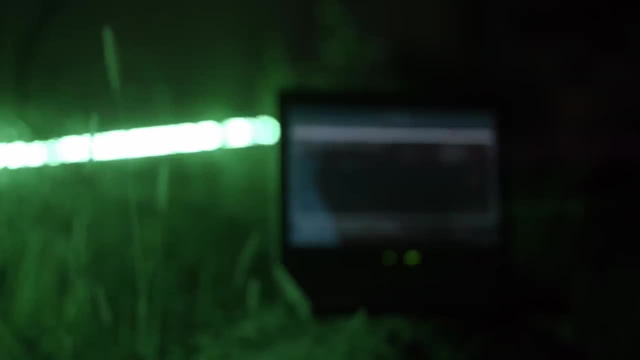 police officer and so on. Very often a weak link in your privacy is not you, but a friend or family member that is not very privacy conscious. A bad actor who's interested in your personal information doesn't have to break the 2048 RSA full drive encryption on your LibriBooted. 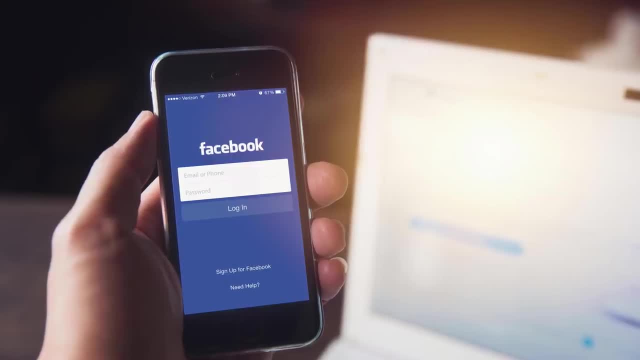 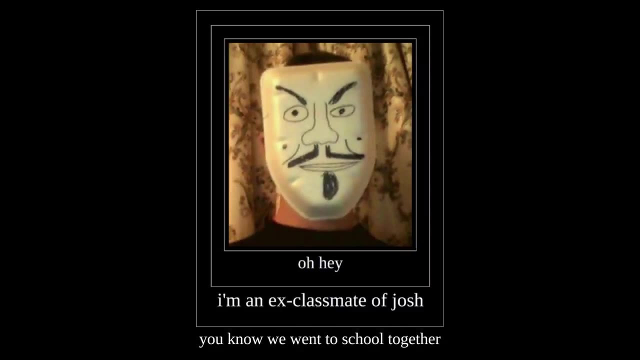 ThinkPad that is running Arch Linux. It's much easier to just create a fake Facebook account and text your grandma or your aunt and say something along the lines of: oh hey, I'm an ex-classmate of Josh. You know, we went to school together, We wanted to meet each other and I just 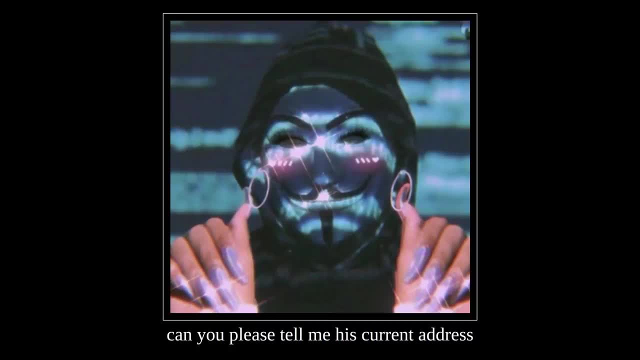 came to town, but he won't pick up his phone. I guess he slept through his alarm. Can you please tell me his current address so I can go and check in on him Now? this might be an exaggerated example, but I'm sure you know at least one family member or friend that you don't want to. 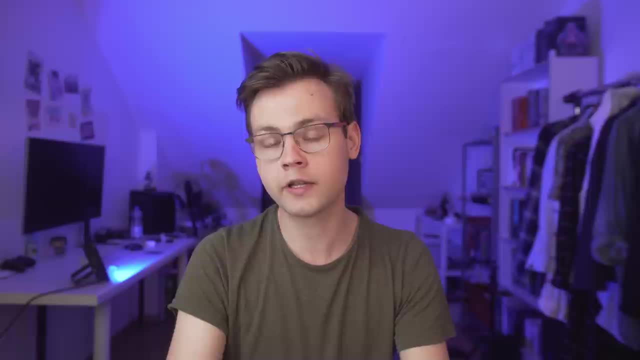 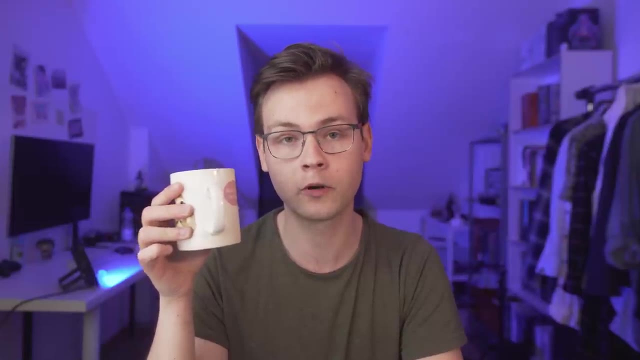 that might fall for this kind of stuff. So yeah, be careful and educate your friends and family. So that's going to be it for this video. I'm sorry for the raspy voice. I have a bunch of water here. I've drank like a gallon of water, but it doesn't help. Anyway, as per usual, 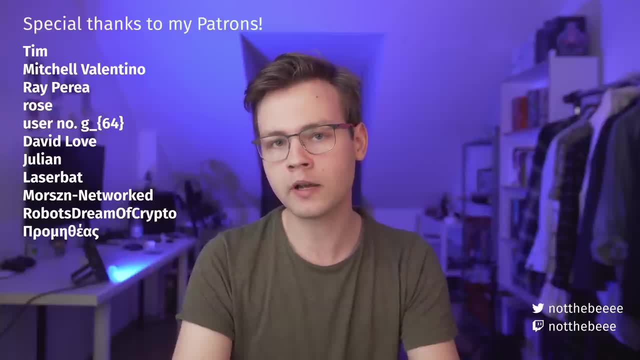 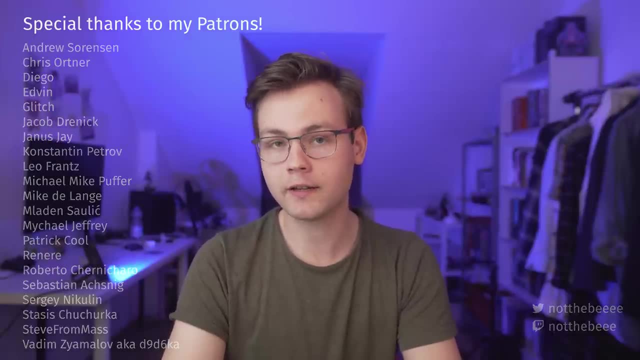 I do want to thank my patrons: Mitchell, Valentino, Ray, Peria, Tim Rose- user number G64, and everyone else who supports this channel. Thank you, guys, for watching once again and I'll see you in the next one. Goodbye.